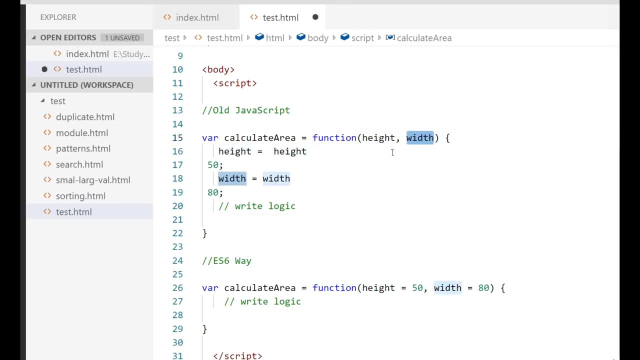 parameters height and width, but we are not able to set the default value here, so we'll have to increase the code and then we do like this. okay, in the previous version of javascript. uh, we have no way to declare- i mean default parameters, like we directly have to pass the parameters and then. 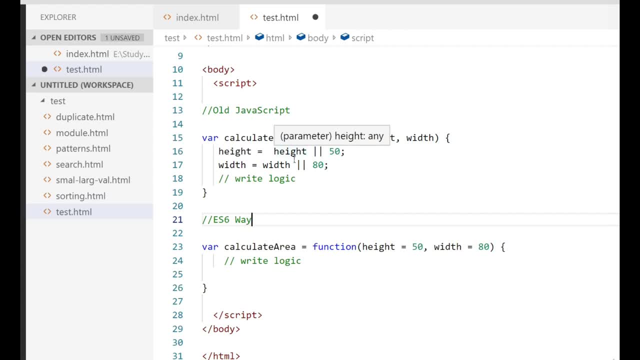 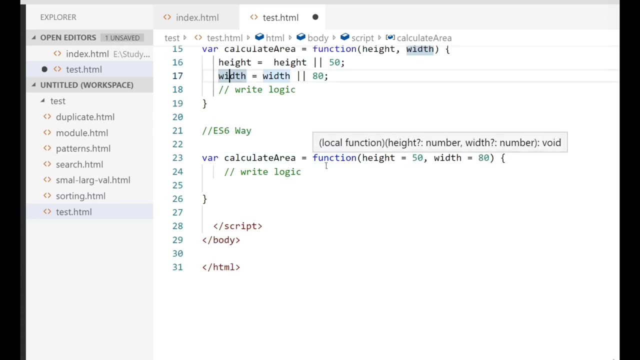 we can write our logic like this: if height is available, then take height, or otherwise take default value, which is 50. so the problem is we have to add two more lines for with the code. but now with the es6 new fa, uh, we have resolved this problem. we got a default declaration of the. 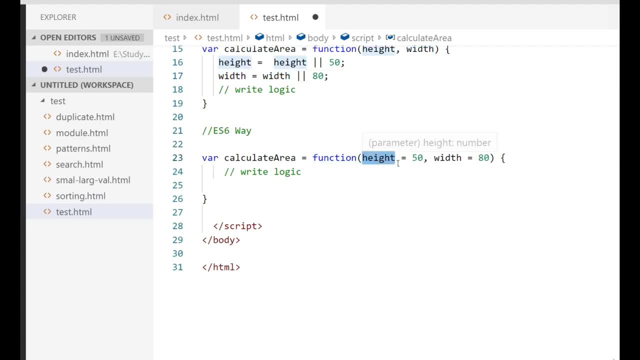 parameter values. so now we can directly pass the default value of the variable. so if the value is available in height, then it will take that one. otherwise it will take the default value, which is the default value of the variable. so if the value is available in height, then it will take. 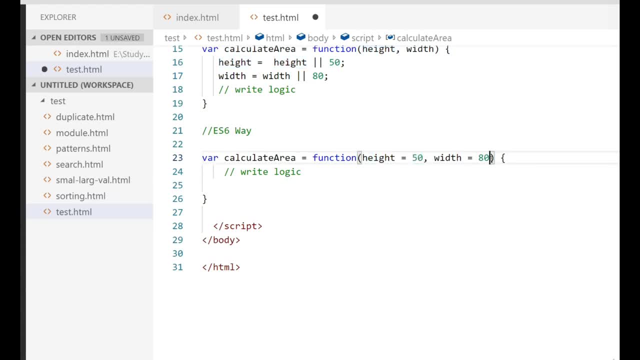 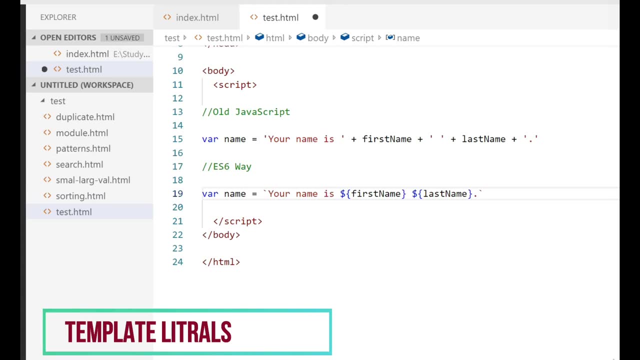 50 and same for the width. so this is the default parameter feature in es6. now let's move to the next feature, which is template literals in es6. so the second feature is template literals. so in es6 we can use a new syntax which is uh, this syntax. we can use this new syntax inside of the. 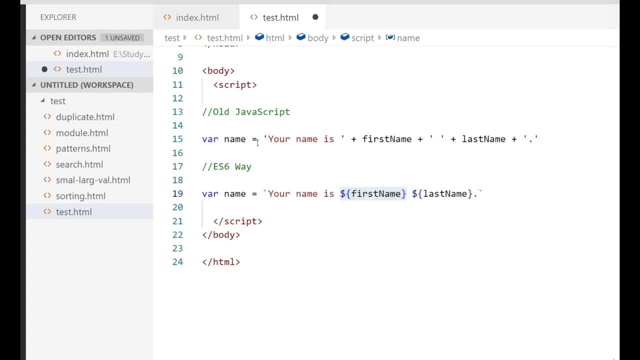 back ticked of a string. so earlier in the old javascript what we have to do is when we have a long string and we want to pass some dynamic value, so we'll have to follow this plus and these single commas and all these things. we have to follow this structure. 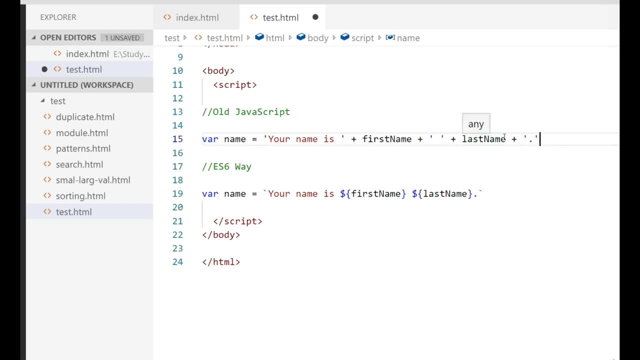 and that is very hectic. basically we have to. every time we'll have to add plus, then we have to start string, then vector plus, then we have to start string. so this thing is a bit complicated but in the new es6 way we have this back tick. this is not a normal string. 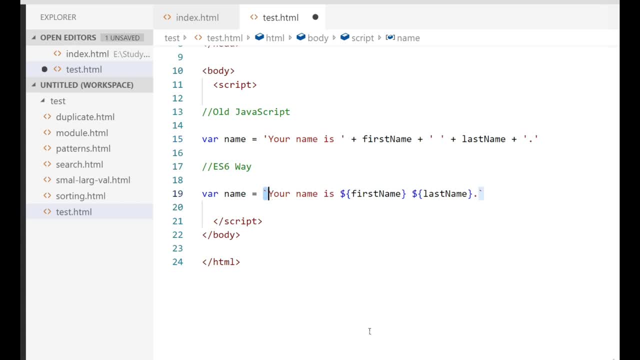 so back tick is what? back tick is simple: uh, the key that is available just down side of escape key. so simply, we can pass one, we can add one tick and we can follow this template, little uh format, and in a single line we can do all our stuff. so this is our templates. so let's 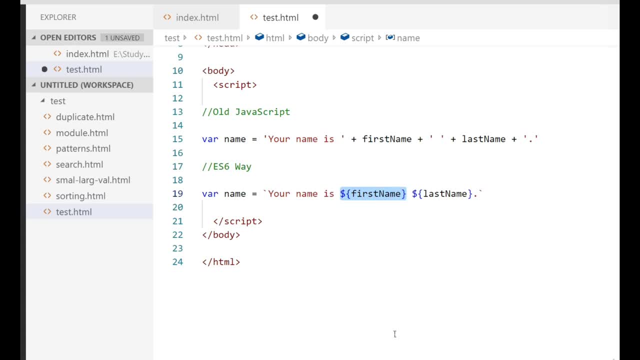 move to our third feature, which is multi-line strings in es6. so let's see how we can implement. so third one, the multi-line string in es6. it is a very cool feature of uh ikmascript 6 because earlier remember uh, we cannot write to sync string and multi-lines if you want to write multiple lines. 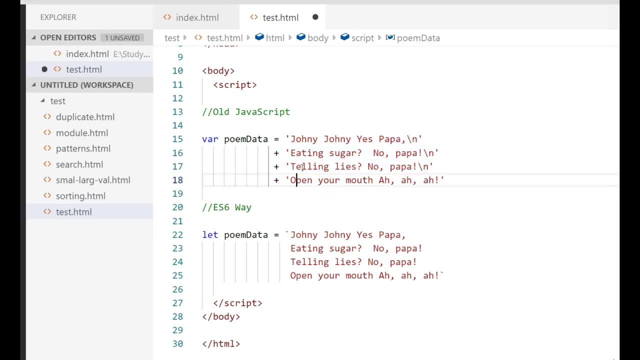 in a string. so we'll have to do this kind of logic, we'll have to write, we have to break string into multiple lines, then add plus, then again add plus and plus. because in a single lines we cannot do that. because if we add, do this in a single lines so we will always start getting lint errors. that 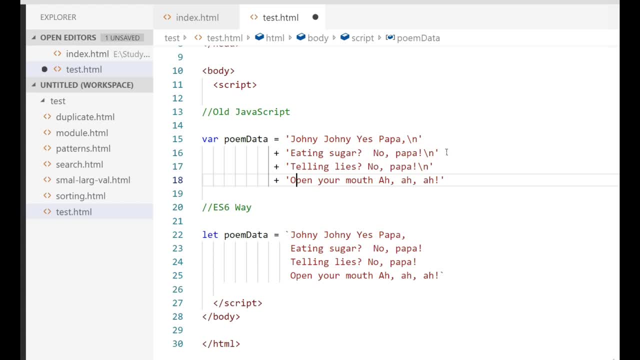 the line length is very long. it is not a standard feature actually. so what we can do is in the es6 way. we just have to use simple this back tick. it's a template string that we have discussed earlier. so simple: add times template string and do whatever you. 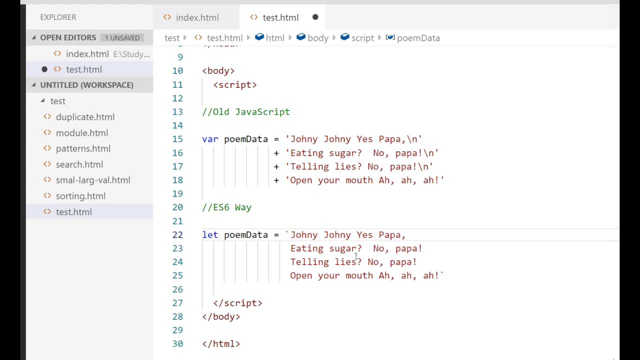 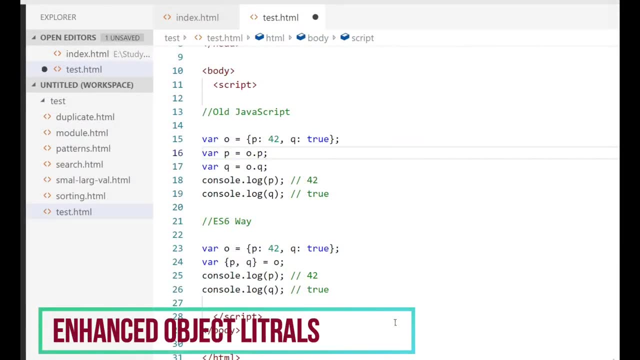 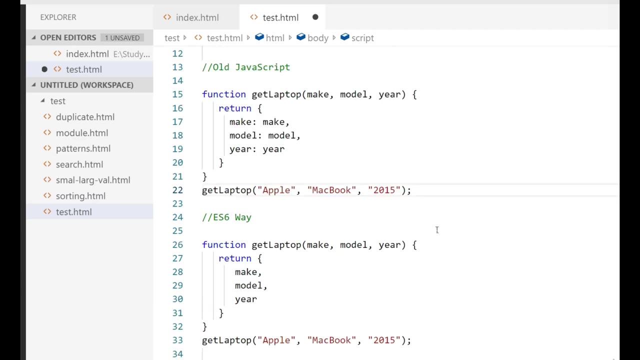 want to do. it will print exactly the same in a multi-line. so that is a very cool feature of javascript, so let's so. now let's discuss about our fifth feature, which is enhanced object literals in es6. okay, so let's do it so by using enhanced object literals in es6. object literals makes it. 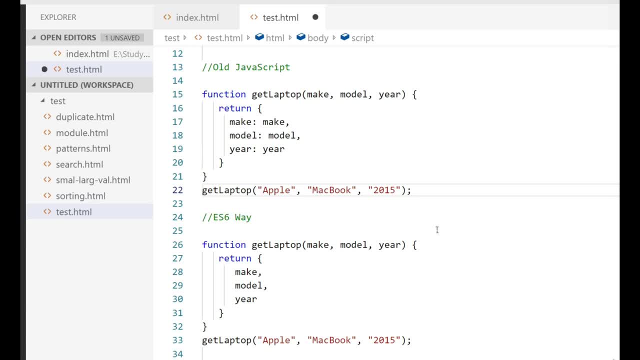 clear that, instead of just adding, we create an object and then, by creating a function within the object, we can quickly create objects with properties inside the curly braces. so let's see how we can do that. so basically, earlier, if we have to return an object from a function or create a 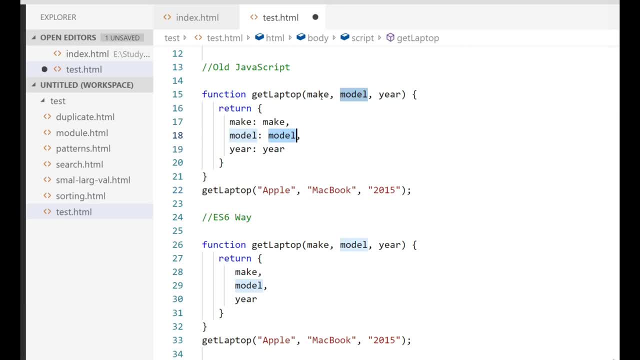 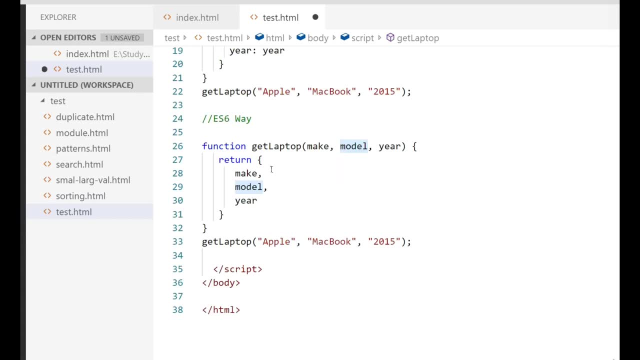 new object. so how we do that? we create an empty object inside that object. we create some property and assign the values. create the property and assign the values. enhanced object- literal feature. we can do by this way. we can reduce our code. what we are doing is we're simply returning these properties inside the 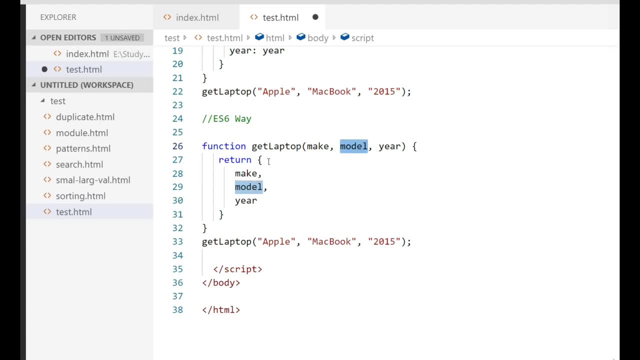 object. so but the name of this property, the object is gonna create, the property name, the same name and the value it is gonna assign to the property. so output will be the same, exactly like this, but it reduced the code. so if you call this function it will gonna always return you to all this property properties. so 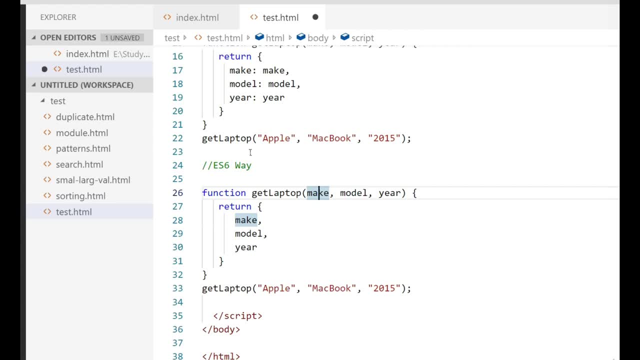 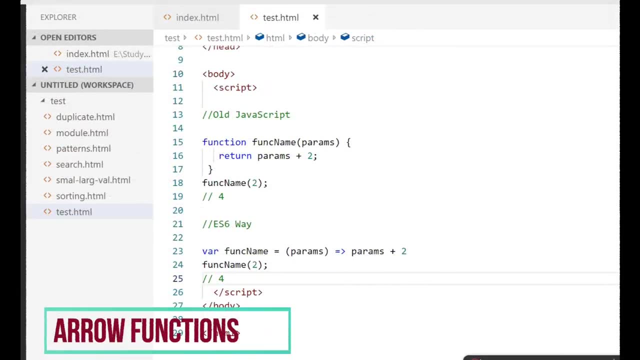 this is how it can reduce our code and we can increase the performance of website if we use it in our code. so the arrow functions gives us a very cool feature. first of all, the syntax wise it is very cool and it will reduce our code and effort. so, first of all, if you will see, the syntax is bit different and bit 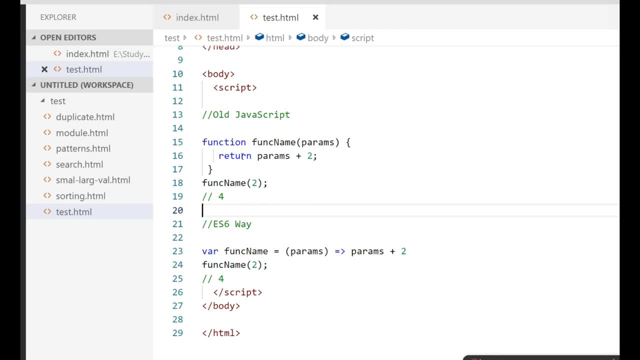 cooler than the normal function. so the normal functions are like this: here we have to write all this function name and parenthesis. we have to add inside that we have to do all this thing. then we are getting over result, but in ES6 way, if our statement is only one single line, like we are just returning. 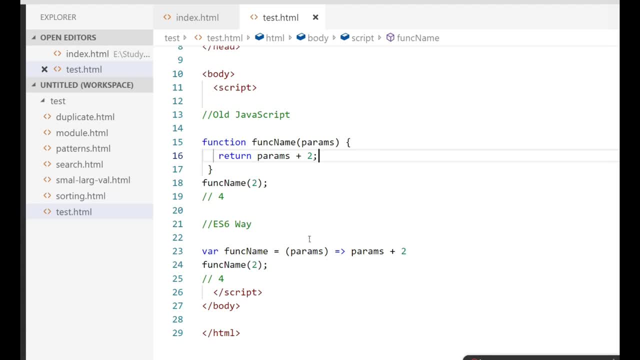 one thing so we can write it down in the one line also, so simple way we can see function, name and parenthesis and we don't have to write this basis of all this stuff in the single line. whatever you are returning, don't have to write a return statement. so we simply can return and we will get the 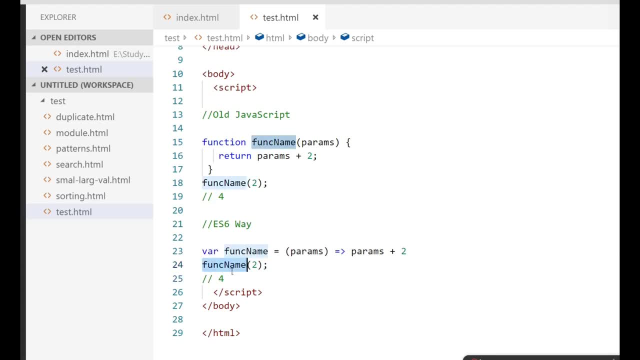 same result when we call this function. so these are basically arrow functions, but also these functions gives us some new features. that is really helpful. like the fat arrow functions would make your this behave properly, because because of this sometimes we stuck into a big problem, so that can help us. so. 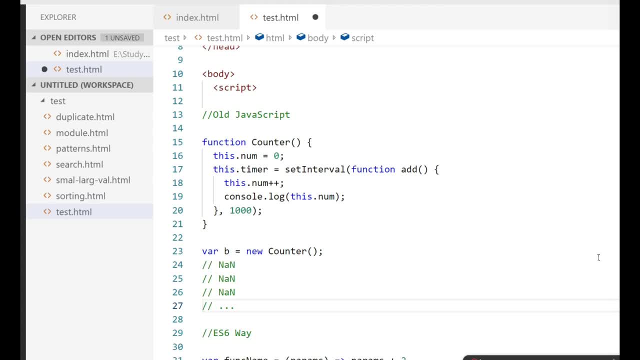 the arrow functions are basically fat arrow functions. unlike a regular function, an arrow function doesn't bind this. instead, this is bound lexically. so what does does it mean? by lexically, that means arrow function always take the scope of its parent functions, so keep it as meaning the original. 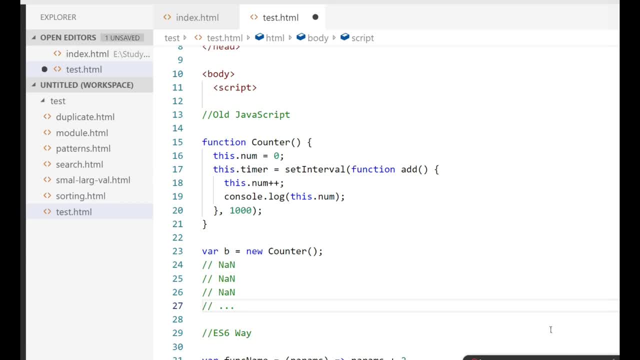 context. so in this example you can see that we have created this function and in this function we have added a. thisnum is zero and we have created a set interval that is gonna increase the number. but if we run this function, so we will get in result: nan, nan, nan, nan nan. every time the 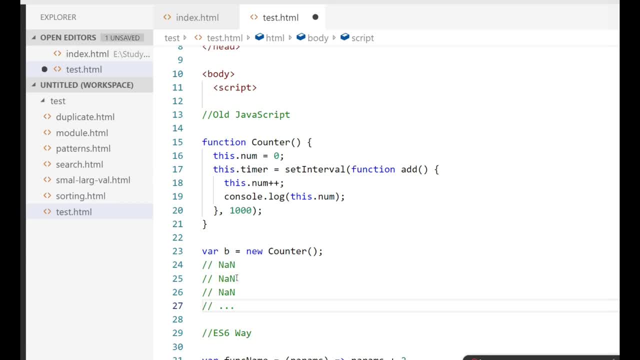 interval will work. so this is the problem that can be resolved by the arrow function, because this problem is offered because of this scope of the normal function, because every function is having its own this. so when we are trying to access this value, the number, the scope code changed in the set interval, it is taking this functions. 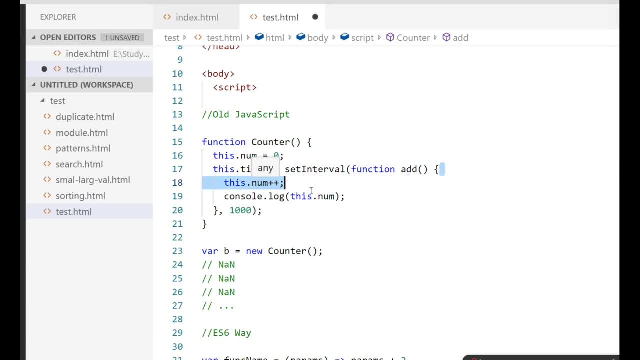 score, and here we don't have any, this number assignment, so it is undefined by default. so when we are going to increase undefined plus plus, it will always gonna return not a number. that is the problem. and now this problem we can solve by using arrow function. so let's see how we can solve. 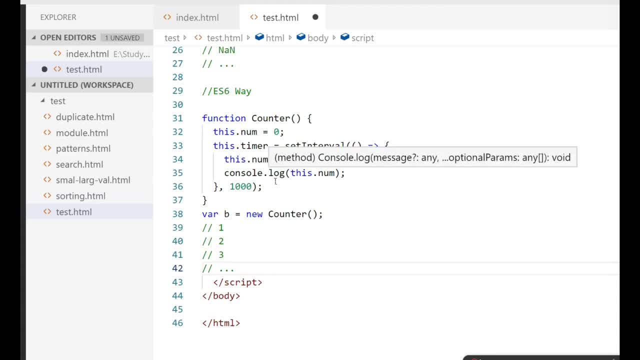 for instance, we. you can see that two squ�리 in between are not the same. so in this function you can see, everything is same, but just we have changed the syntax of the function. we made certain travel by using arrow function. so previous you guys, previously you can see that we are using normal. 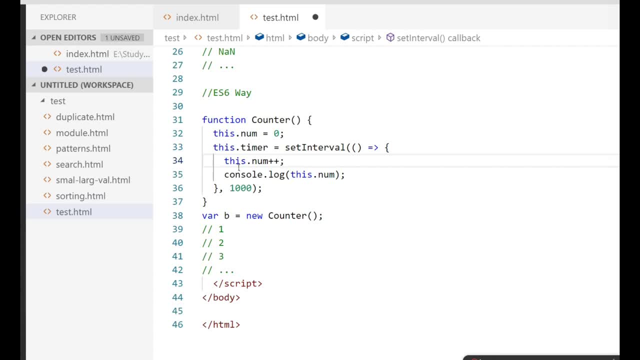 function, but here now we are using simple andł function, which is basically a non-numous function of arrow. so in this function what it is doing is it is equal to this number. okay, so the thing is it was always gonna take 0 here, and 0 plus plus is 1, 2, 3, and it will goes on. so this is how we solve this problem. 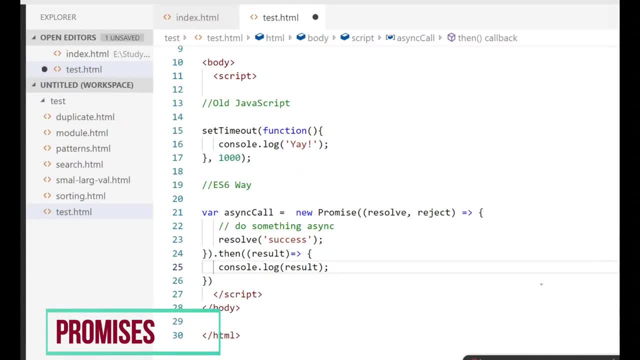 okay, promises are the new feature of ES6. so what are promises? promises, basically, that we used to handle our synchronous responses earlier in ES4. what we have, I mean ES5, what we have, we have simply callback methods, and callback methods are always having some problems, if you are aware about callback. 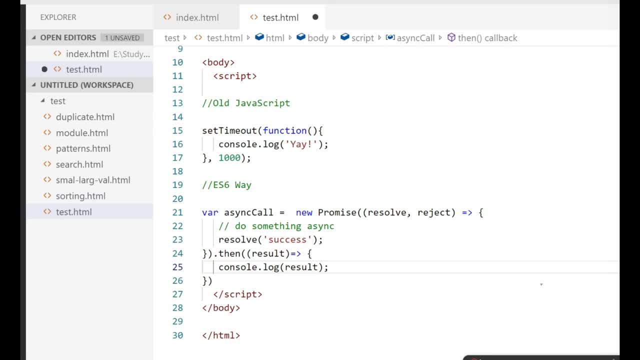 handling situation. so JavaScript provided us this promises to resolve that problem. so in ES6 we can use promises with arrow functions. so here you can see that example. so what we are trying to do is we have created a new promise that will return us a resolve or reject. so in our 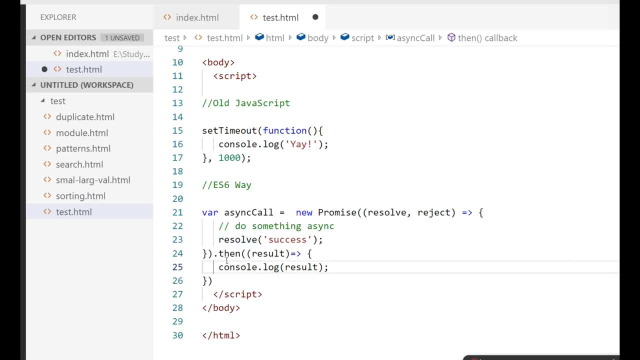 case it is returning Resolve and we have to pass some values that we can access with the then method. so once this promise got success and it will return the resolve, with this value and with the help of then method, we can get this value and we can do whatever we want to do here. we are simply consoling. 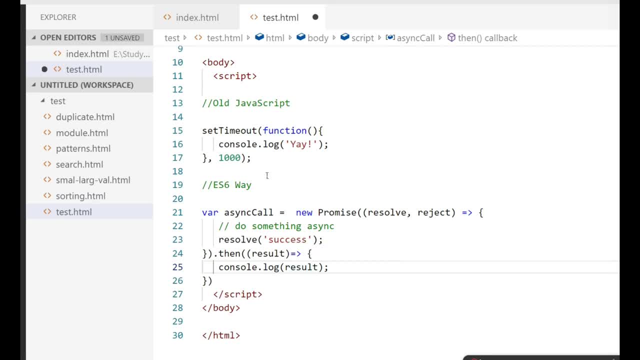 this result, but in ES5 earlier. we don't have promises, so we'll have to use this set amount of things for asynchronous things, or we have to use callbacks. so, as we know, callbacks always have some problems, like callback hell. if you are aware about this, if you are not, 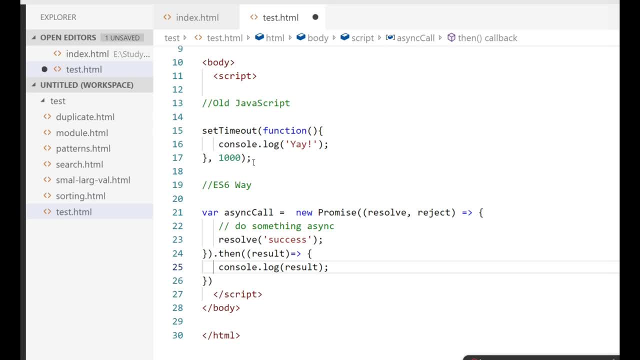 aware about this, then i have created a separate tutorial, separate tutorials, on callback. i will add the link in the comment. you can go there and you can watch. so this is all about promises and if you want to learn in into deep about promises, so i will also create a new tutorial. tutorial on 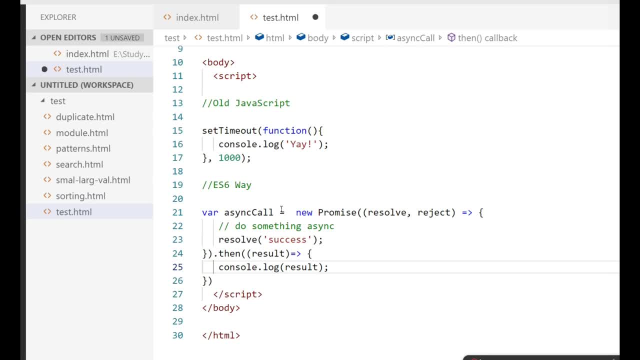 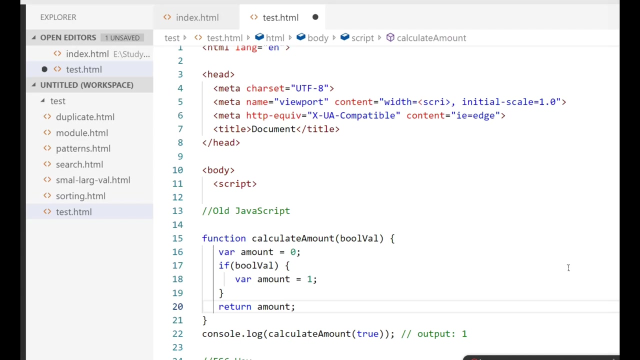 promises separately so you can watch it and let's move to our new feature of es6, which is a very important feature and the name is block scope constructor and which is latent scope. so let's continue on that. so, first of all, uh, what are block scoped variables? so in javascript, es6- 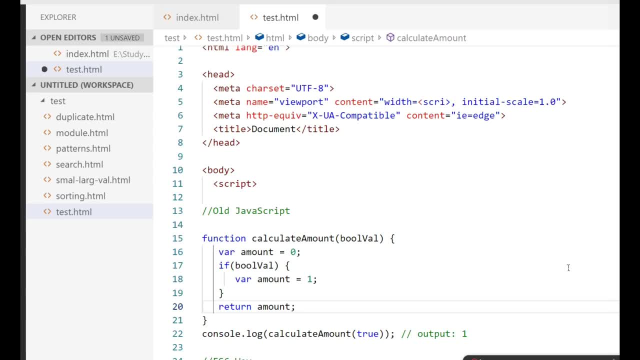 has introduced two new variables, which is let and const. so let is a new variable which allows to scope the variable to the blocks. so the main difference between let and variable is: variable is scoped to the nearest function block and lat is scoped to the nearest enclosing block which can be smaller than a function block. and another thing is variable. 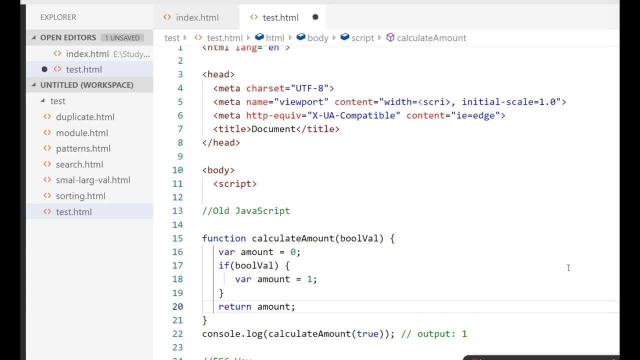 always got hoist, but the lat and const never hoist. so if you want to learn more about what is hoisting, i have created a separate tutorial tutorial on that and I will have added a link. you can go there and you can watch what is hosting in JavaScript. so, for short, hosting is something whenever. 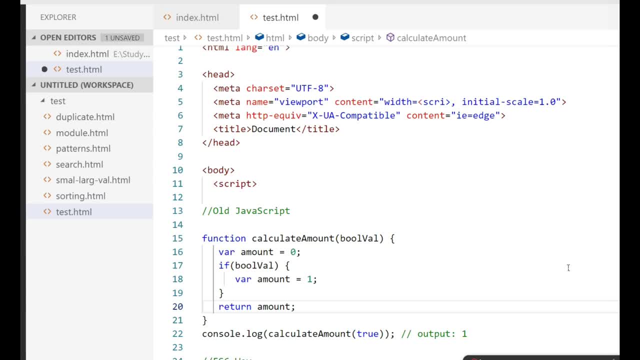 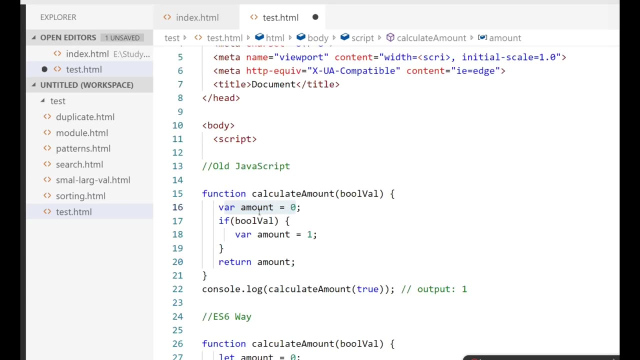 JavaScript compiler runs, it always housed the functions and variable on the top of the function scope. in JavaScript we have two types of scope: one is global scope and second one is function scope. okay, so in this example you can see that we have variable amount in this function, which is 0, and inside this condition we 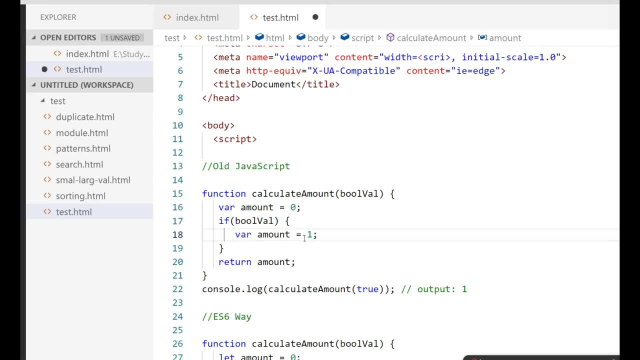 have created another variable which is equal to 1. that means this amount is going to host on the top the global scope, and first it is gonna take the value 0. once this condition is goes true, it will go and update the same variable with the one. so now we have written two variable differently, but at the top, at 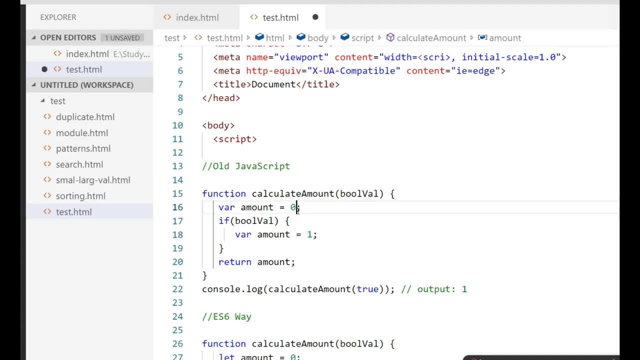 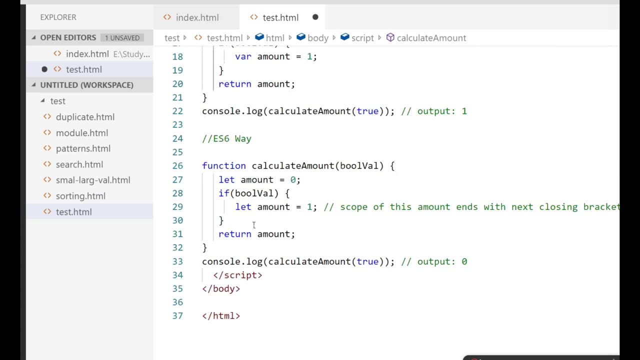 the time of hosting, it will gonna merge into one and it is gonna update this value from 0 to 1. so at the end, when we return this amount by this function, it will always return output 1. but this is for variable, the normal variable that JavaScript have. but in the case of let, if you will see, 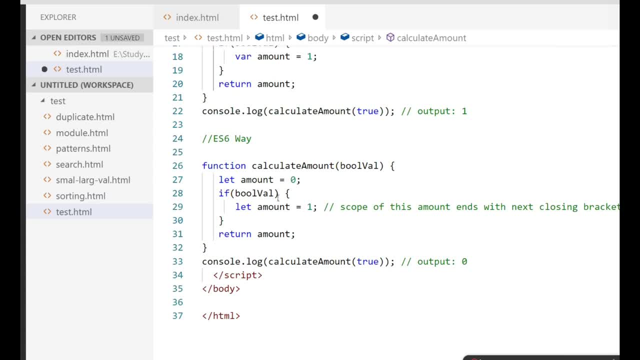 we have two lets here, similar as variable. okay, but this let scope is only inside this function and after that we have created another if condition. in the inside if condition we have created another amount variable with the let and we have updated the value, but the scope of this let only this if condition and it doesn't. 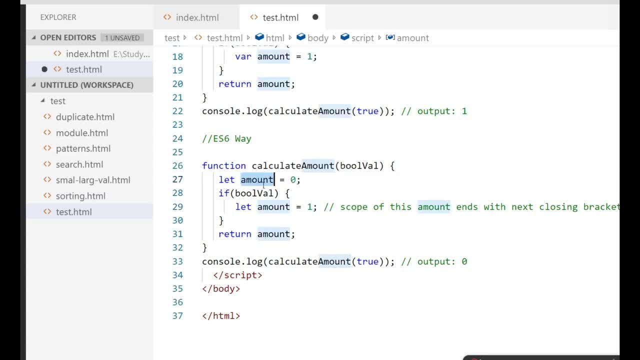 host. so it is not gonna update the value of this amount, so it is. it will always gonna return you 0 because it is not going inside and it has created its own separate block scope. so we have two amount having different properties values. so, simply, we are returning this amount and it is pointing to this amount. 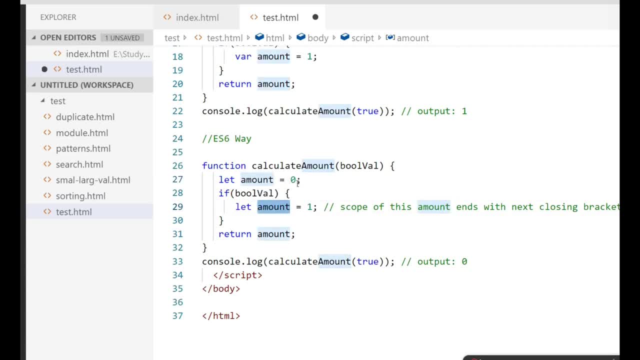 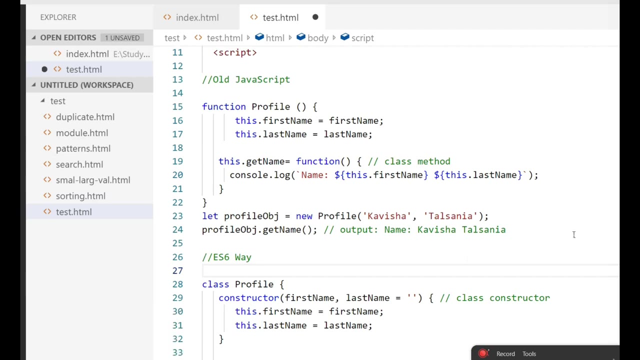 only not this amount, because it is not updating the value of 0 because of block scope. it is all about let and const. let's move to our next feature. okay, so now we are going to discuss about the ninth feature of ES6, of our tutorial, which is: 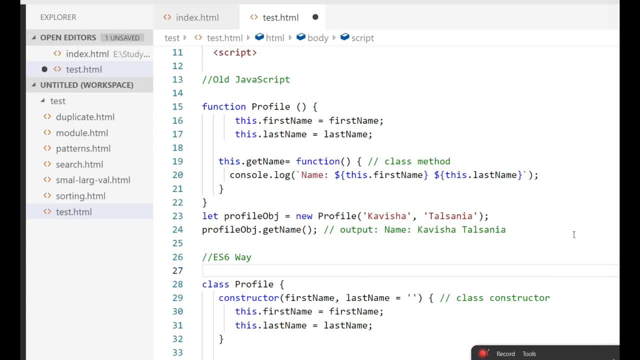 classes. classes are the very important feature of ES6. it is nothing, just a constructor function. and they just added a synthetical sugar on the constructor function and and I'm renamed it as a class. so now we can see with our code examples how we can do. 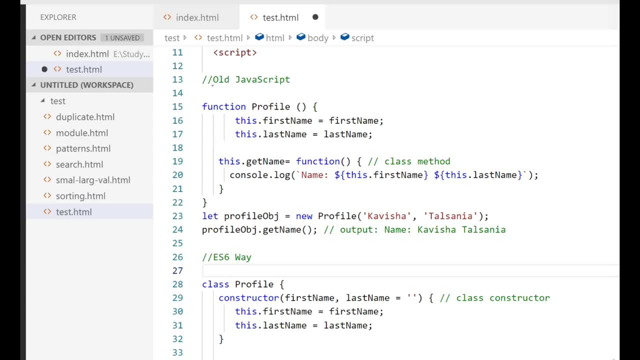 this. so here we can see this code as written in ES5, the old way. so in this construction function, what we are doing is we simple created a construction function, inside that we have created some properties and a function, and after that we get it an object via new keyword and pass some values and the 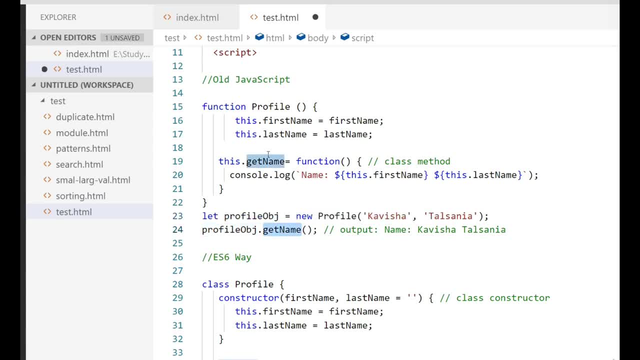 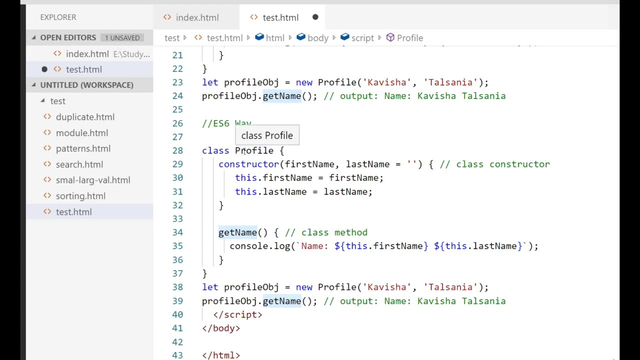 help of this object and we can directly call this function. so simply, we just created a constructor function and after that we get it a new object of this constructor and we are using it. but now in ES6, how we can do this same code like this: Instead of using constructor function name, we use class name and the syntax is like simple: 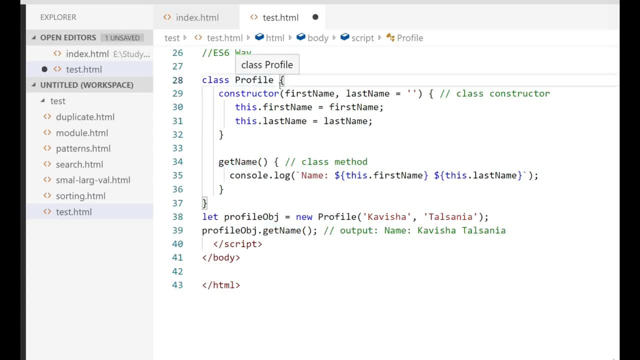 object. We don't use this parenthesis here. So according to the rule in the syntax, every class have a constructor method. So constructor method is going to receive two properties and this is going to take default properties empty. If nothing is there, then empty string that we just have discussed earlier in this session. 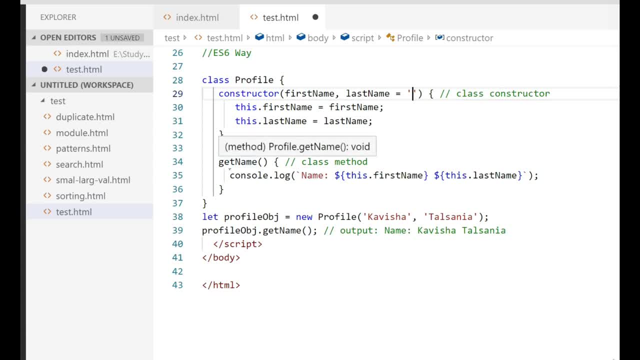 And after that we just simply the code is same. This is the syntax of written function inside the class. We don't have to use the function keyword and everything. We simply write the function name and parenthesis and start code And after that all the process is same. 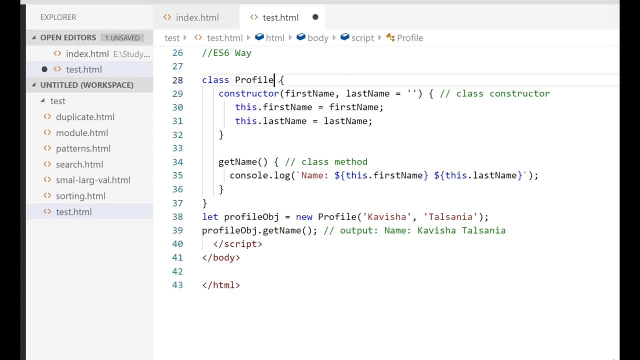 But only the class thing is: function constructor has been replaced by the class name. So that's all for classes. Nothing new, Or, if you want to learn in detail about classes. so I have a separate tutorial for the same. also, I have added the link into the description. 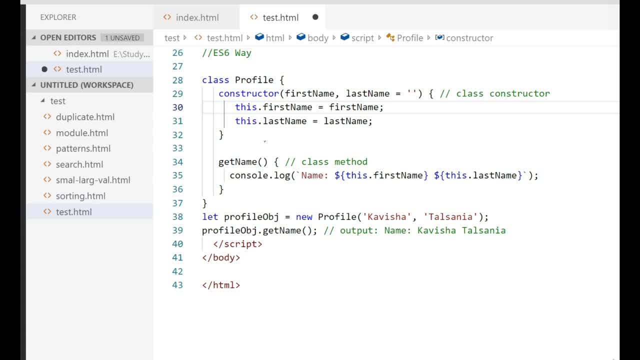 So you can go from there and you can watch the complete class tutorial in detail, So you will better get to know what are classes. Okay, so that's all for classes in this session, And now let's discuss about the last 10th picture of ES6 of this tutorial. 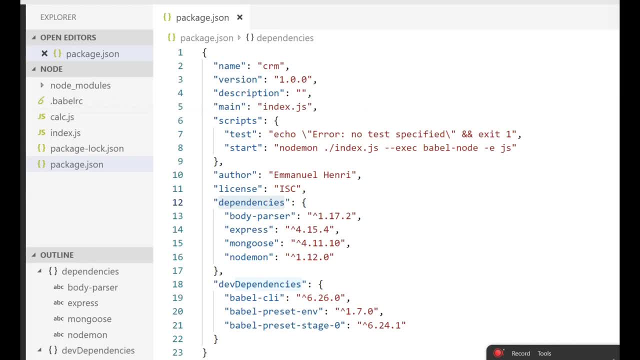 Thank you All right, Okay, So in this section we are going to discuss about the modules that are the 10th feature of our class, That is, the most important topic of ES6. And the module is something it's kind of architecture, basically the main use of this architecture. 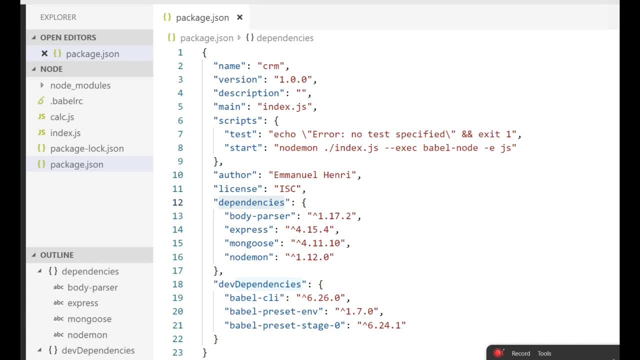 we can reduce the duplication of the code. we create a particular module and we can use it multiple times. So that is the main concept of creating modules. So now modules. The main features are like: we can create a module, then we export this and that we can. 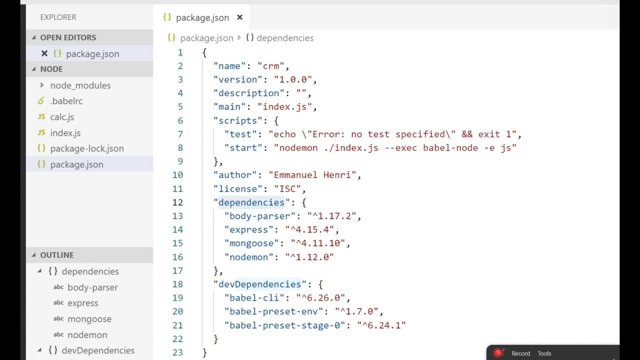 import in other files And directly we can use the same code of the module into the other files. So that means we are saving our code, we are not doing duplication. So this is how we can use practically. So here you can see that I have this folder, which is a node folder. 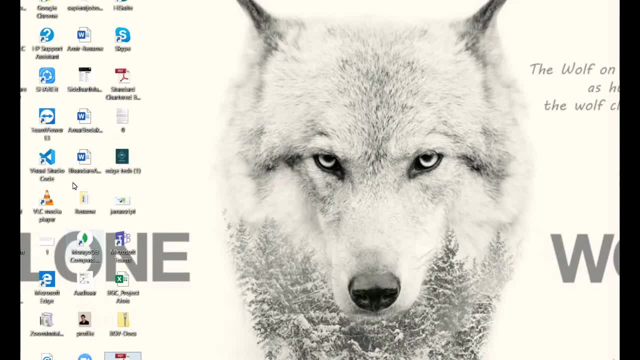 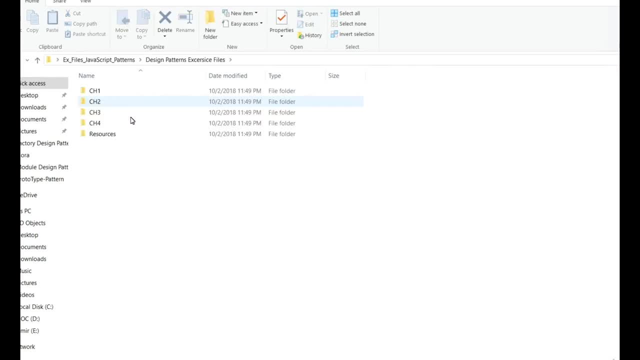 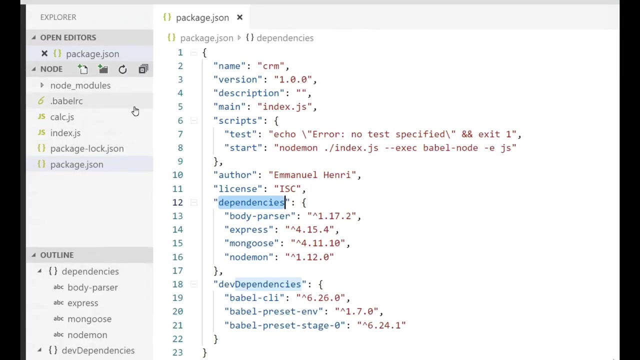 And this folder is: This is the code, This is the code. This is the code. So this is the code. Alright, so in this folder, if you download this folder, you will see the resources. Inside the resources, you will see the node folder. you just have to open this folder. 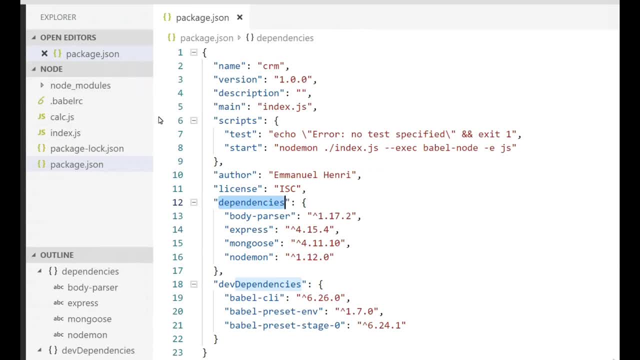 into your IDE. After that you have to open CMD And terminal of this folder And directly. so after once you done with installation, you will get all this module inside the node module section. that is the requirement of the application, and make sure you have installed Babel. okay, some for some users. you will see that this: 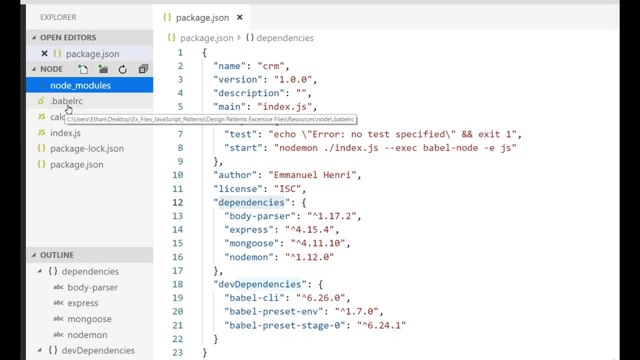 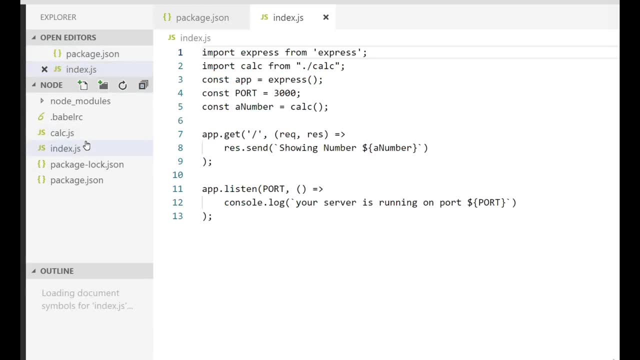 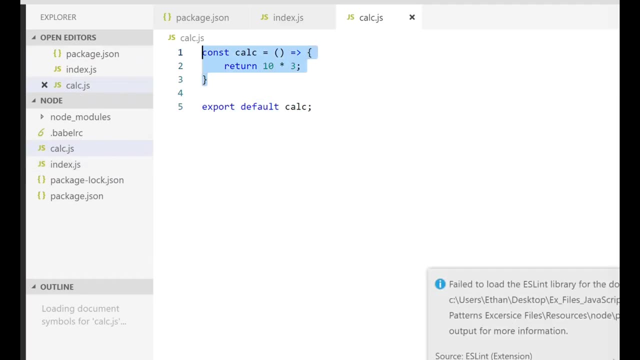 thing is hidden because of your settings of the system. so make sure you have installed Babel also, and in this file I have indexjs and calcjs. so what I have done is I have created a simple calculator that is going to calculate two values and it is going to return that result, and after that I have just 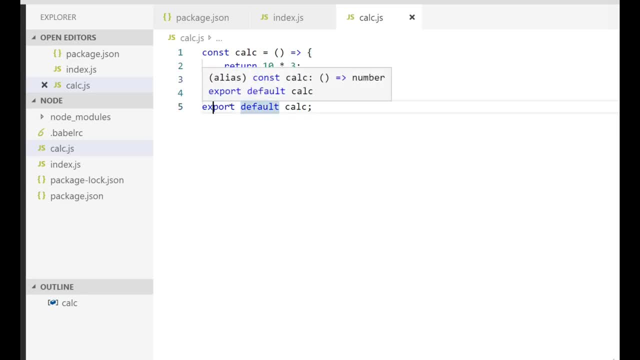 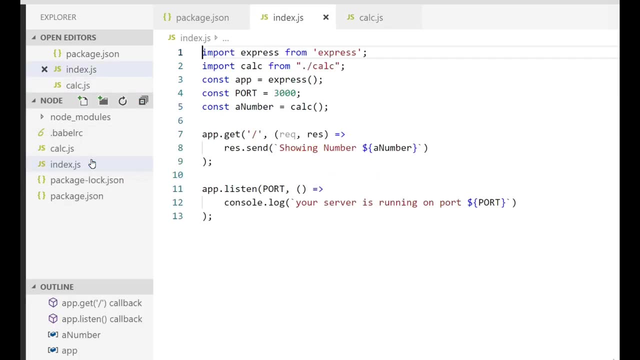 exported this calculator method. okay, that means it can be accessible inside all the application. if I export something- and now what we are doing is in indexjs- I just simply import this and I have used this calc method and signed to a number and I'm simply printing this number inside this. okay, so this is how. 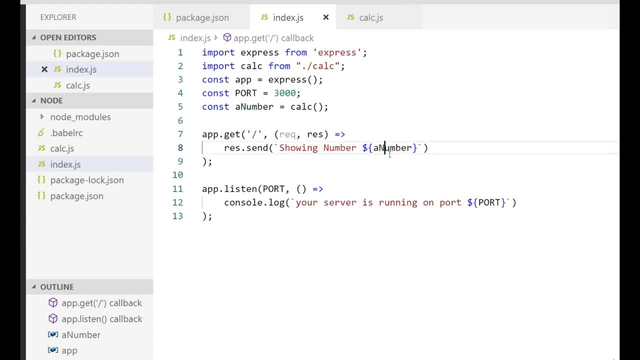 I'm using. so I just want to use this number value here. but I have created it at a common place and exported this so I can use it anywhere in the application. so this is how module works. I have created a module, exported it by import. I can.